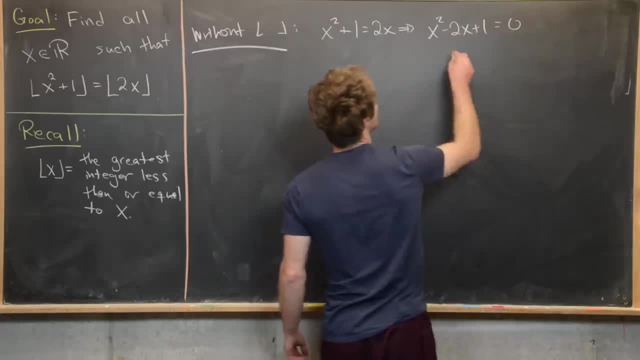 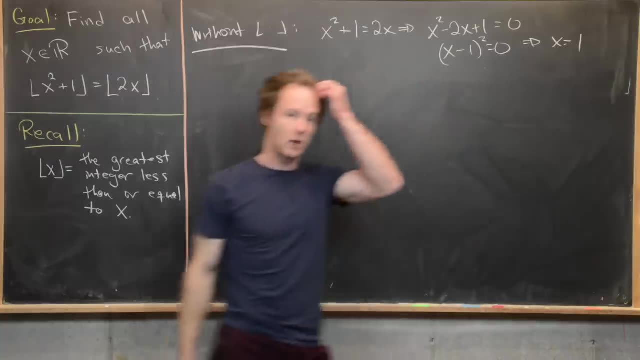 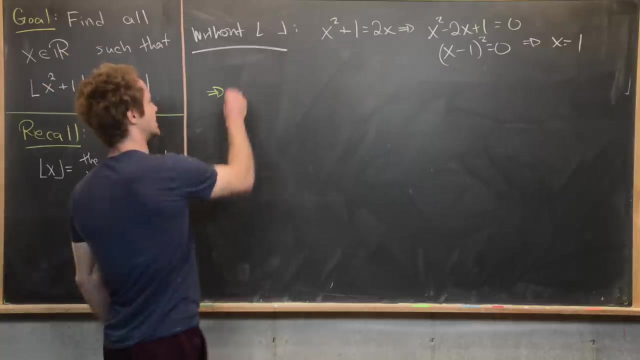 as x squared minus two, x plus one equals zero. But that nicely. factors like x minus one squared equals zero, which tells us that x equals one is the only solution without the floor. So that gives us some motivation for our solution, And by our solution. 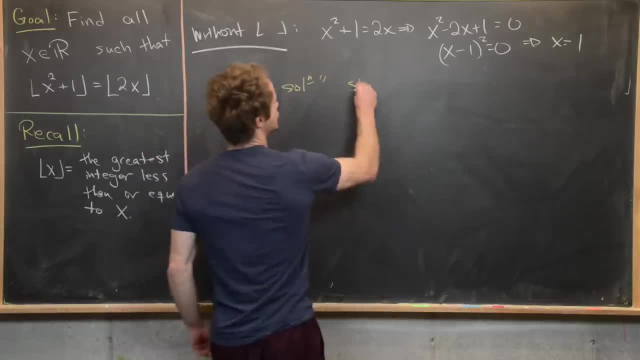 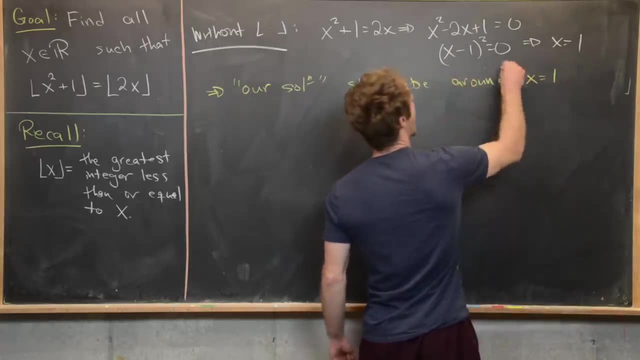 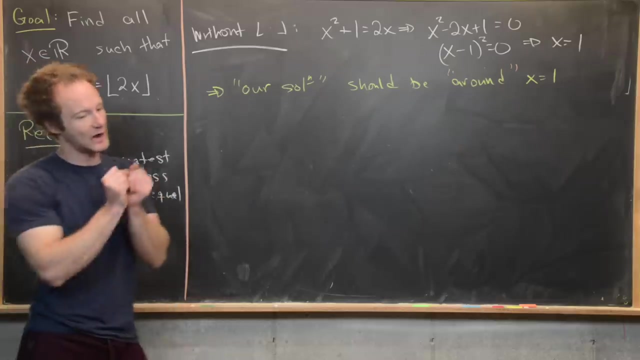 I mean the one that involves the floor function should be around x equals one, And I'm gonna put in quotes around because I'm not gonna carefully define that or anything. Okay, So now what we wanna do is examine what happens if we're far away from x equals one. 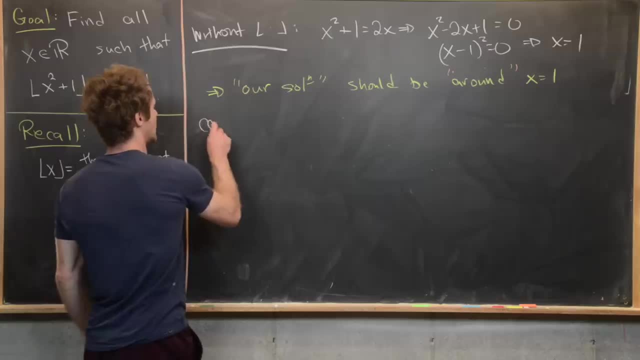 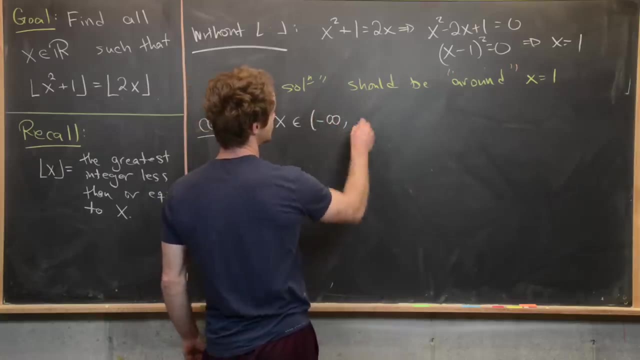 and show there are no solutions there. So maybe we'll break this into cases. So case number one will be: x is in the open interval minus infinity to one half, And then maybe it's an open interval on the side of one half as well. 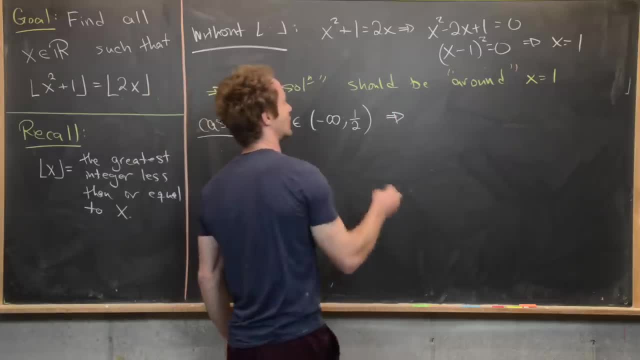 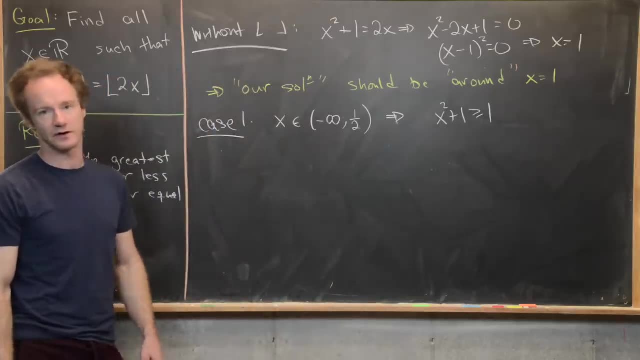 So what I wanna notice here is that we have x squared plus one is gonna be bigger than or equal to one. In fact, x squared plus one is always bigger than or equal to one, But that tells us that the floor of x squared plus one. 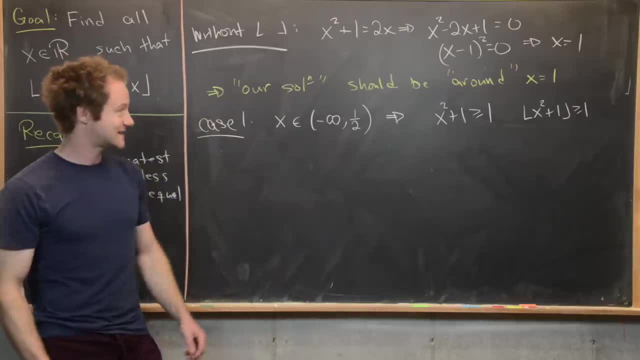 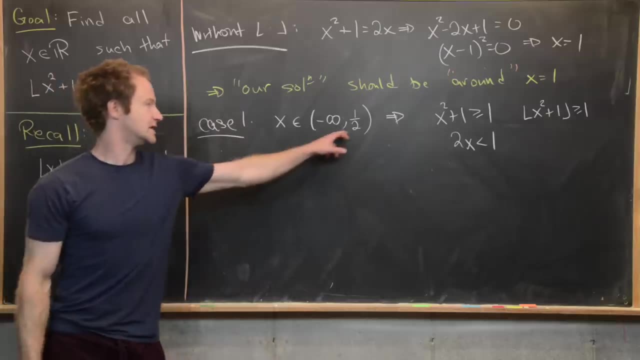 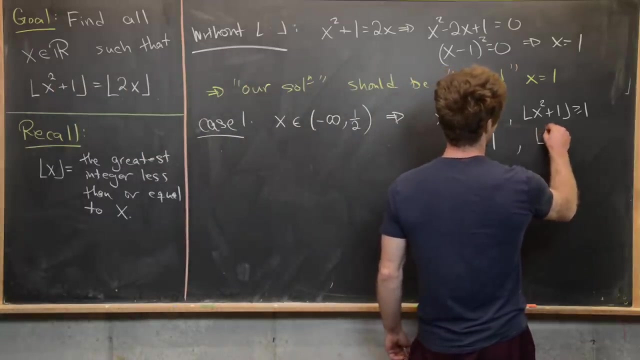 is bigger than or equal to one. But with this setup we have two times, x is strictly less than one because we're not including half in the upper bound for this interval. But what that means is that the floor of two x is less than or equal to zero. 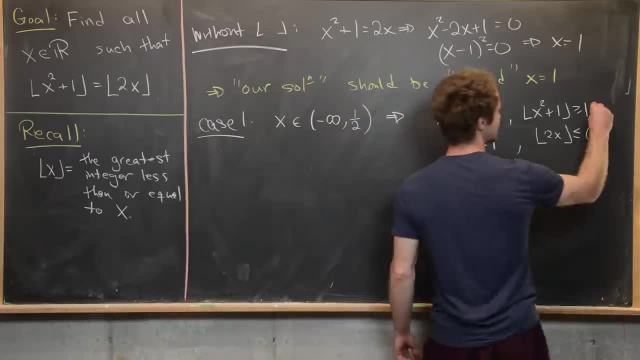 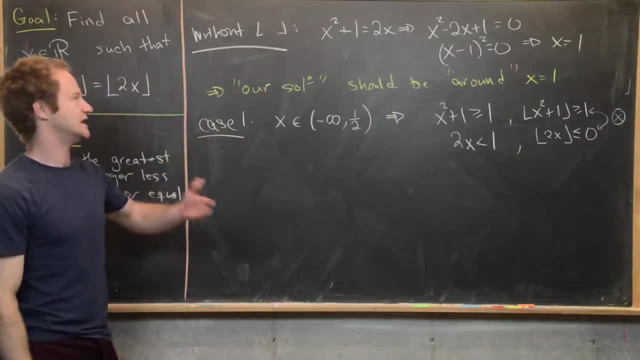 But now what we wanna notice is that these two conditions are incompatible, So it's impossible to have equality there, And that's what we need. We would need equality there for that to work out. So we've got no solutions in this interval. 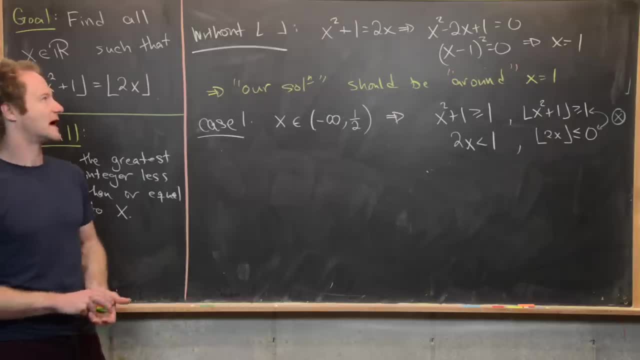 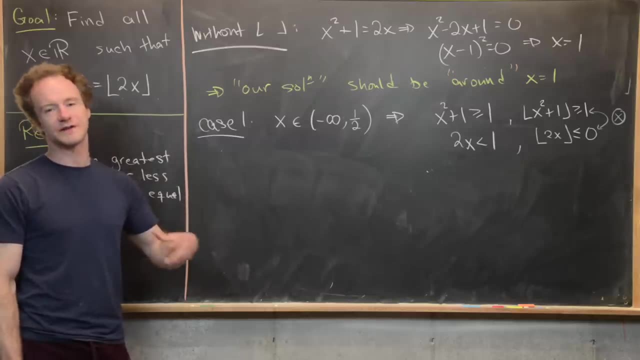 minus infinity to half. So now we wanna be inspired by the fact that if you take two squared and two times two, you get the same thing. But for all values of x bigger than two, taking the square is gonna give you something appreciable. 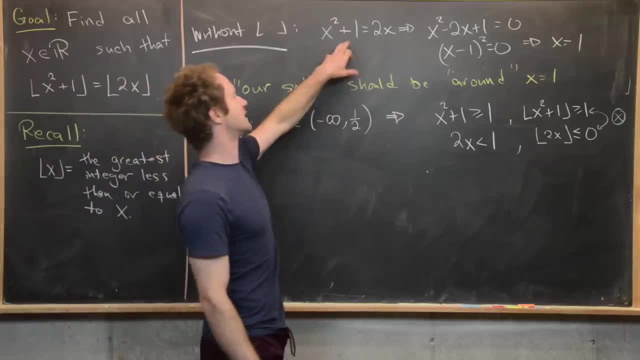 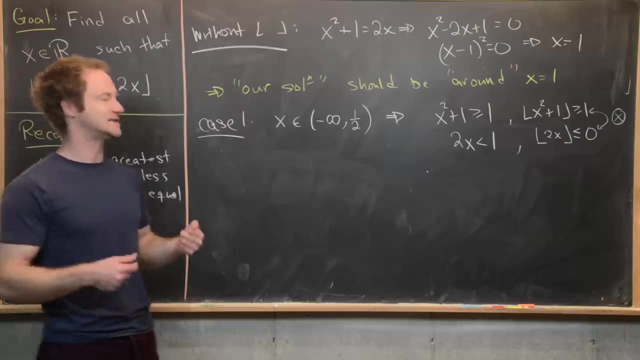 So that tells you that when x is bigger than two, this thing on the left is gonna dominate that thing on the right. So that's not a very careful way of doing it, but that does give some intuition for our next case. So our next case. 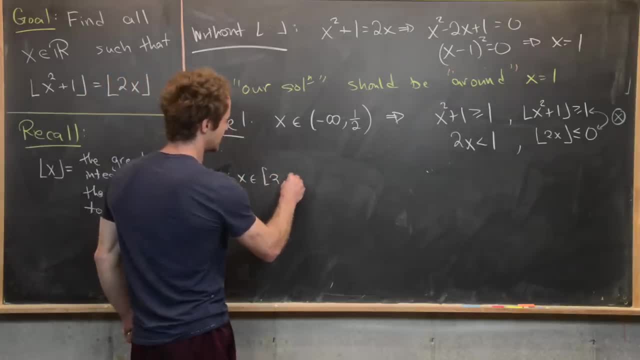 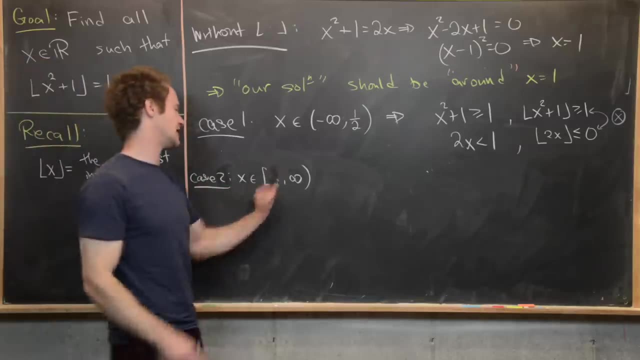 so case two, that'll be, x is in the interval two to infinity, So including two. Now what I wanna do is place x between two consecutive integers in this interval. So let's do that, So we can write two, two, two. 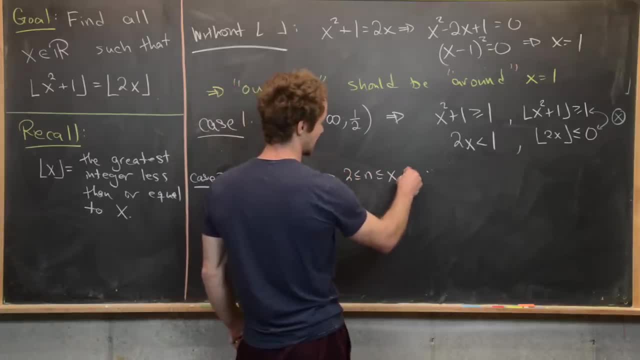 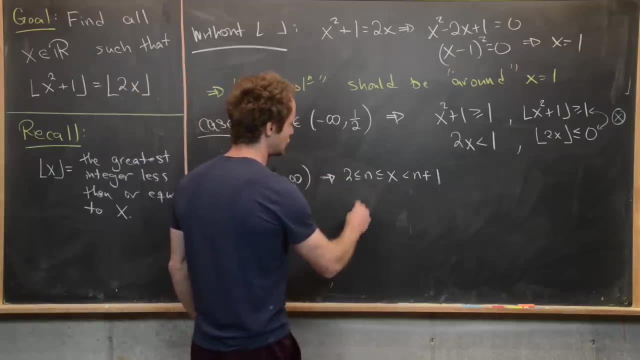 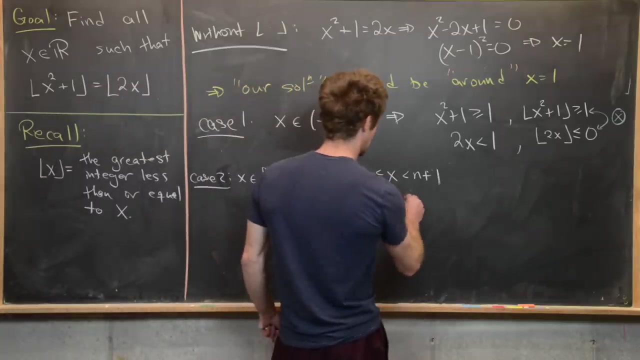 So two is less than or equal to n, which is less than or equal to x, which is strictly less than n plus one Great. But now notice that that means that two x is between two n which is bigger than or equal to four. 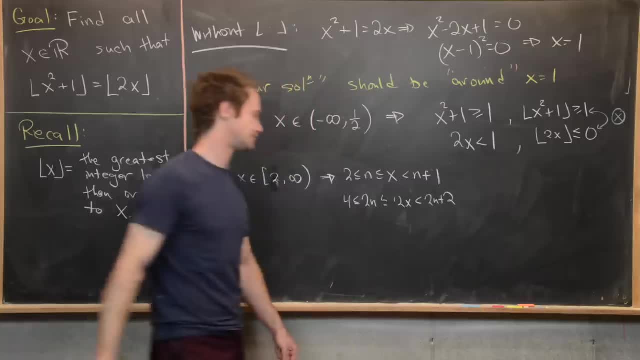 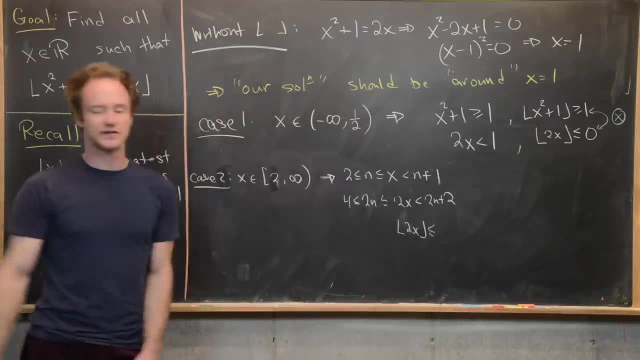 and then strictly less than two n plus two. But now, if we take the floor of two x, we can change this non-strict inequality to a strict inequality with two n plus one here, and then we still have two n over here. So notice, including two n. 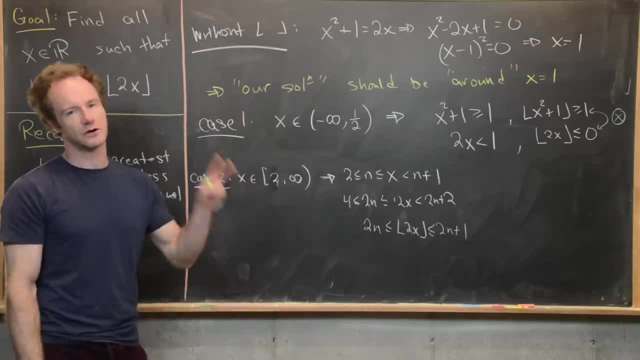 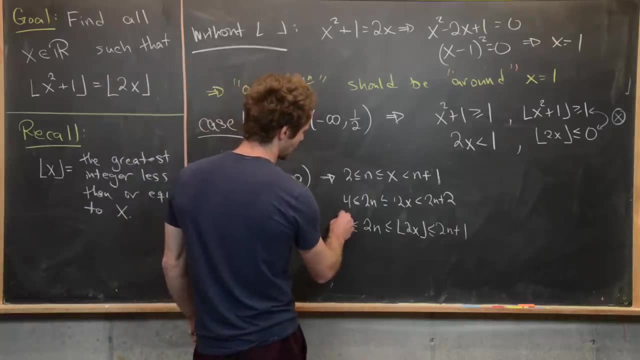 between two n and two n plus two. not including two n plus two, there are only two integers: two n and two n plus one. So those are the values that this floor of two x can take. And then over here we still have this four. 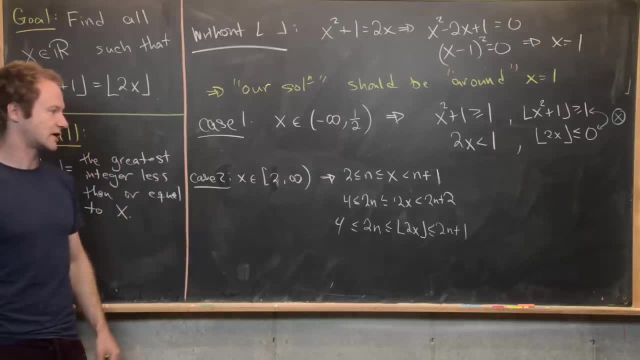 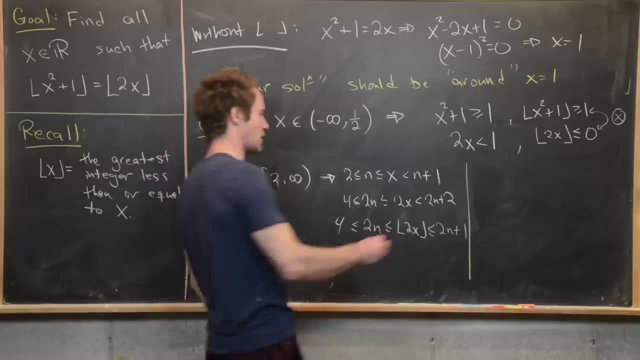 Great. Now the next thing that we're gonna do is do a very similar calculation, but on our quadratic portion. So we're gonna do a very similar calculation, but on our quadratic portion of this equation, But now we can square all sides of this inequality. 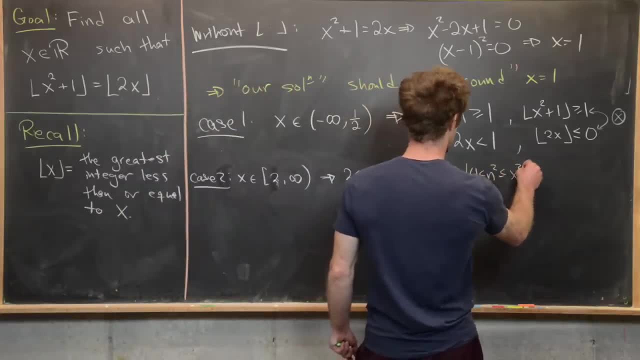 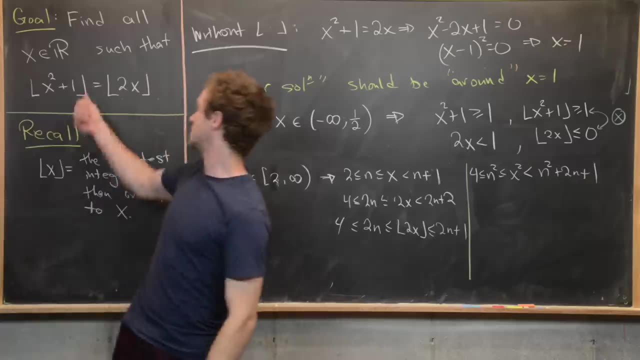 and we'll have four: is less than or equal to n squared, which is less than or equal to x squared, which is strictly less than n squared plus two. n plus one. Now we'll add one to it to achieve this quadratic expression, right here. 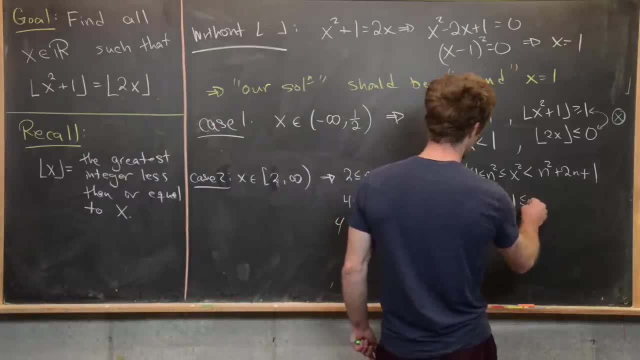 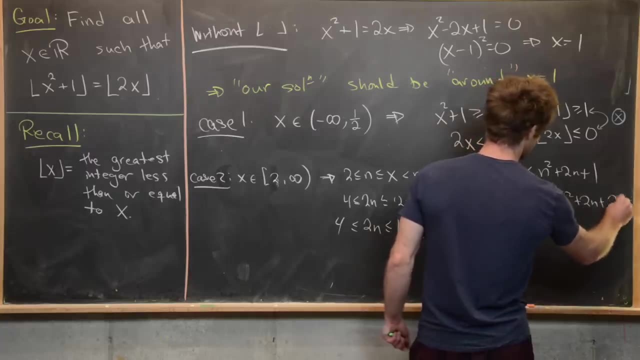 So we'll have five is less than or equal to n squared plus one. which is less than or equal to x squared plus one. which is less than n squared plus two: n plus two. Good, Now I can go ahead and take the floor of both sides. 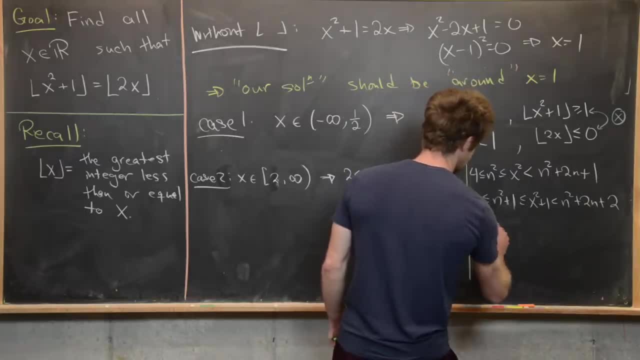 Notice: taking the floor of all sides of this, I'll get five is less than or equal to n squared plus one which is less than or equal to the floor of x plus one, or x squared plus one which is less than or equal to the floor of this. 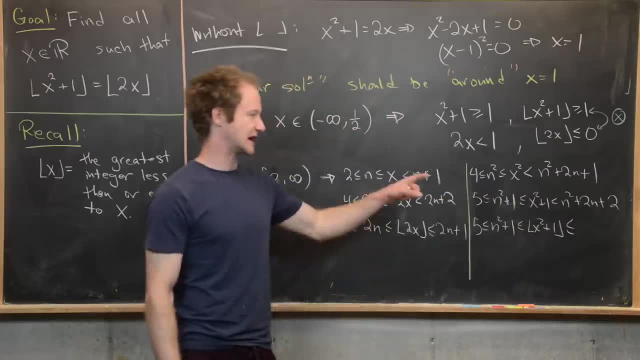 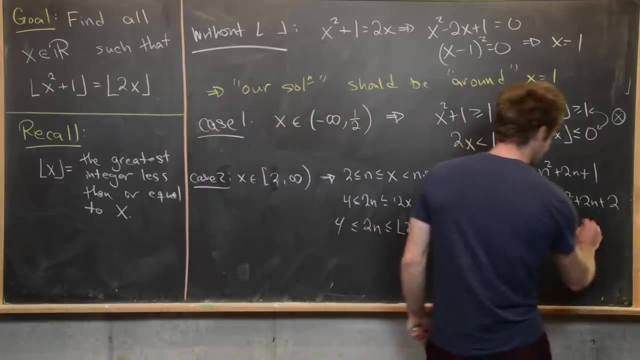 but this is an integer. But since we have a non-strict inequality, we can exchange it with a strict inequality by looking at n squared plus two, n plus two, n plus one, But that's the same thing as n plus one quantity squared. 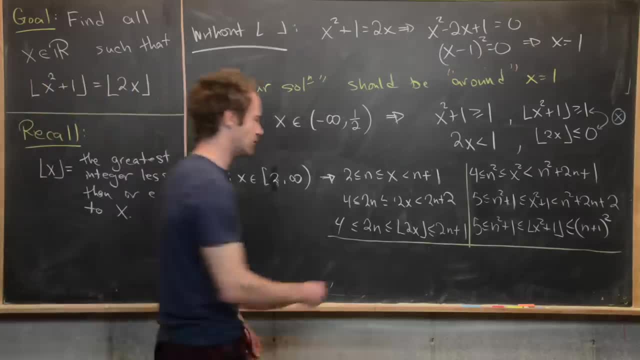 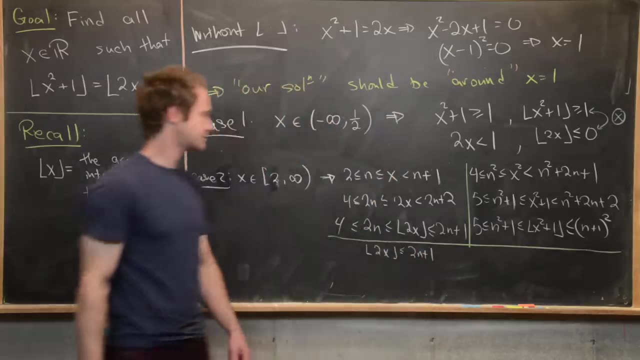 So now we're gonna put these two inequalities together and that's gonna give us something pretty helpful. So we'll have the floor of two x over here. That's gonna be less than or equal to two: n plus one. But notice if n is bigger than or equal to two. 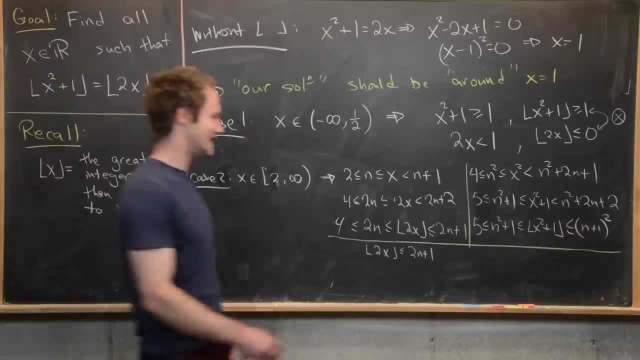 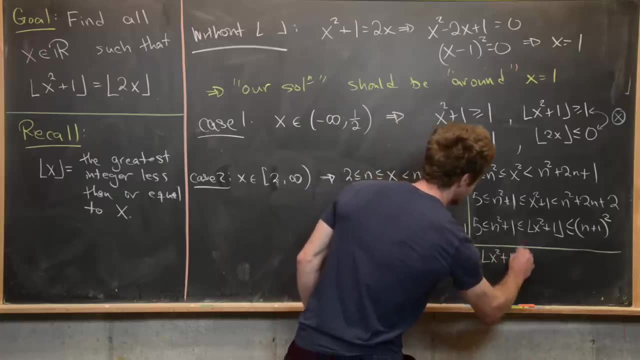 we know that two times n is going to be less than or equal to n squared. So we can put a less than or equal to n squared plus one which is less than or equal to n squared plus one which is less than or equal to the floor of x squared plus one. 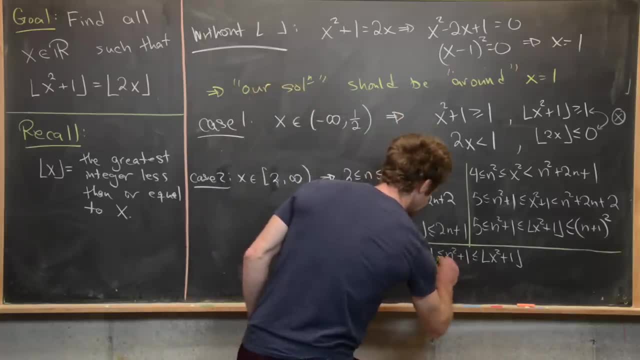 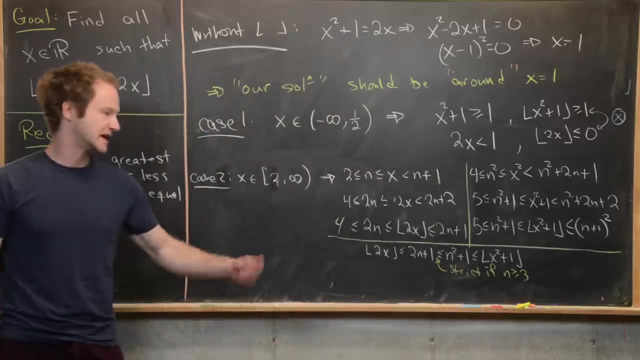 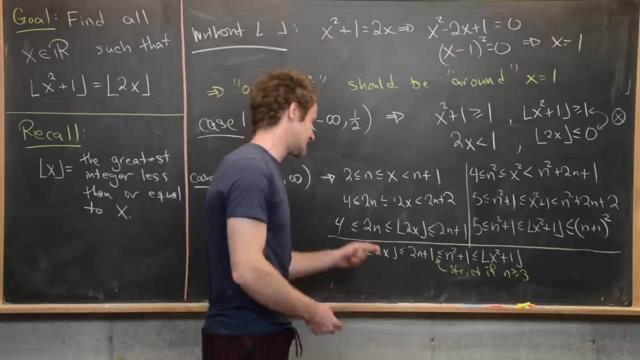 And now another thing that I wanna notice is: this is strict if n is bigger than or equal to three, because n squared is gonna be strictly bigger than two n if n is bigger than or equal to three. So what that tells us is that we've got a strict inequality. 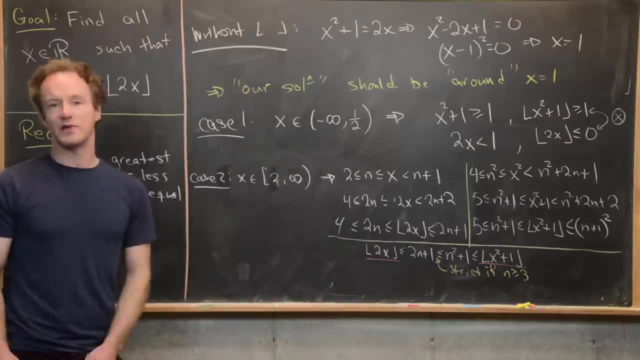 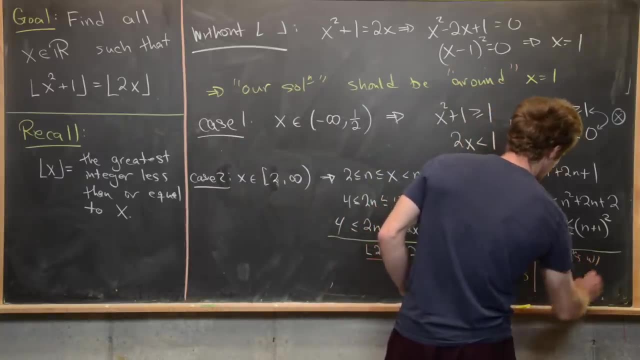 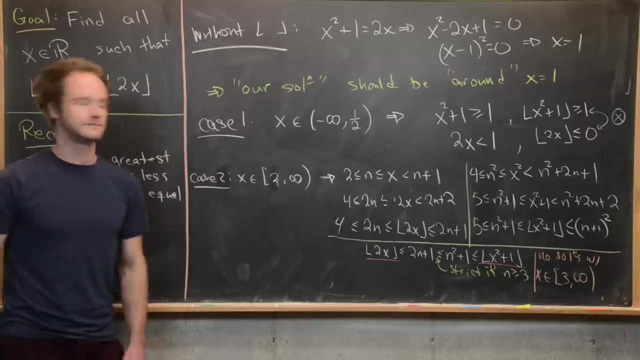 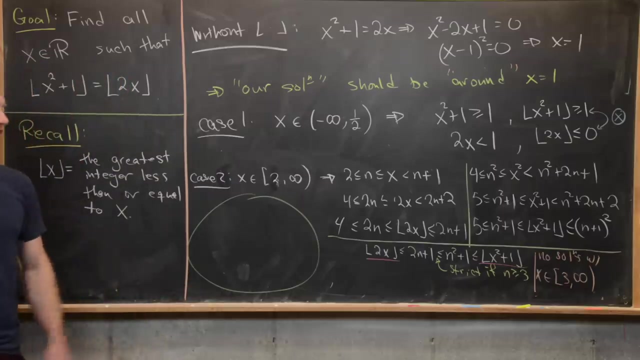 between the two sides of our equation for n bigger than or equal to three. so immediately we see that there are no solutions with x in the closed interval. three to infinity. Good, and now maybe as a little exercise for yourself, that means that we need to check the interval. 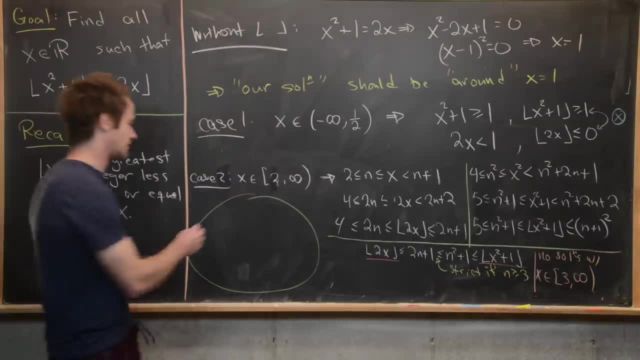 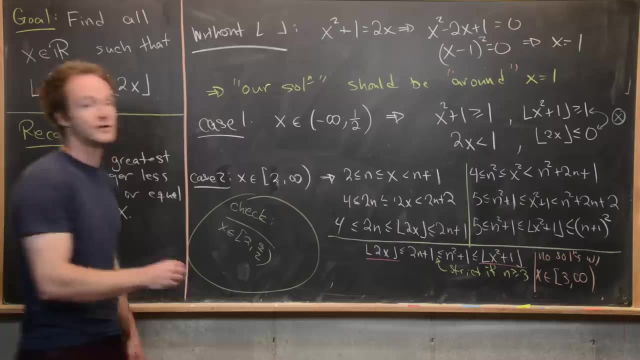 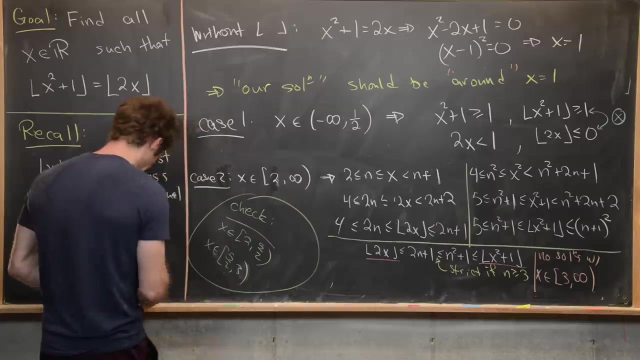 between two and three, kind of by itself. So I would say: let's check this x in the interval two to two a half, you'll see that you'll maybe want to break it up into pieces. and then x from two and a half to three, and you'll see that there are no solutions in this case either. so that means there's no. 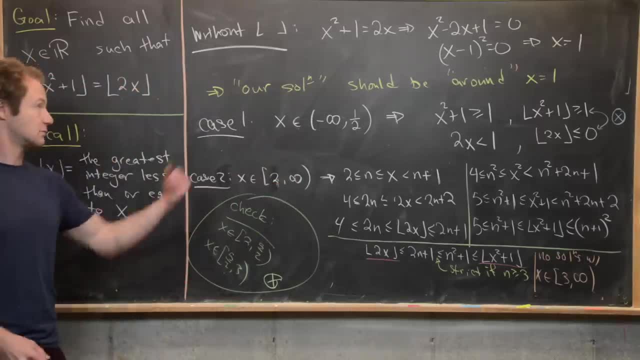 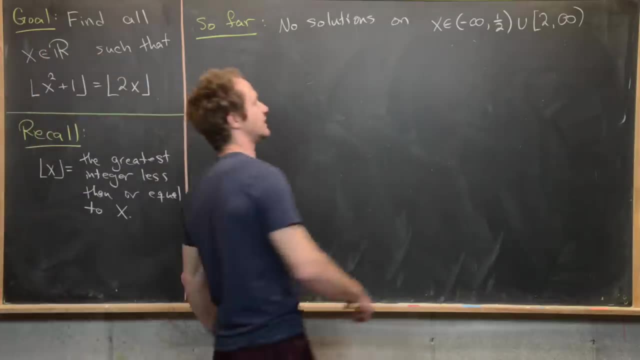 solutions here. no solutions here. now we're gonna maybe clean this up and then we'll start looking for where there are solutions. so far, we've proven that there are no solutions on this. union of intervals minus infinity to half. union two to infinity: we do not include a half, but we do include. 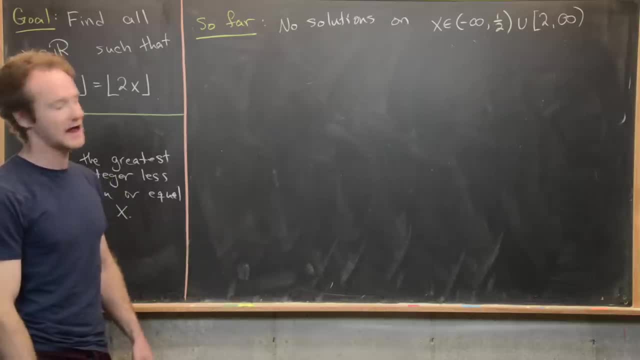 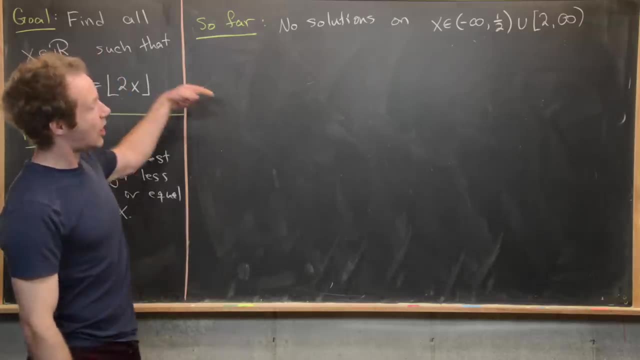 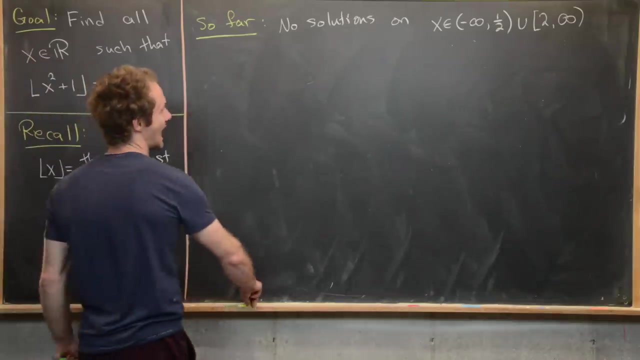 two, in fact, as you can see, we'll check that one half will give us a solution. okay, great. so now the next thing that we want to do is look at all of the cases in between one half and two, and this may seem like maybe too big of a problem, but, as we'll see, it's not too bad if we break it up. 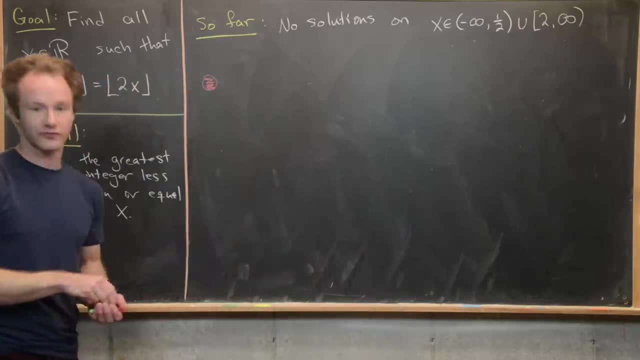 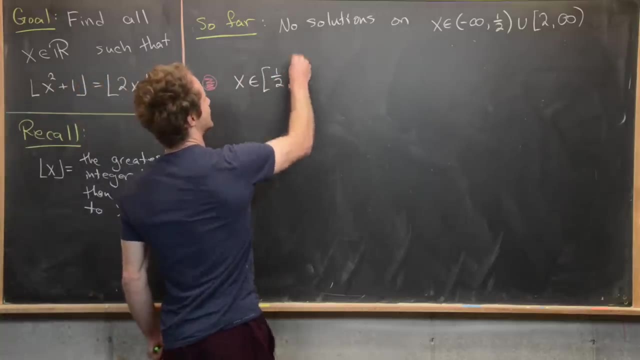 carefully. so let's go ahead and break it up. we'll break it up into three cases, and so that first one will be: x is in the interval one half to one. so closed interval on the left, open interval on the right. and you might say, well, what's the point of this choice? well, notice, if x is on this closed interval, that means that two x. 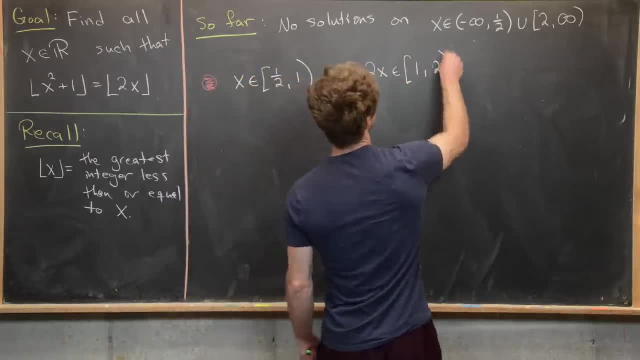 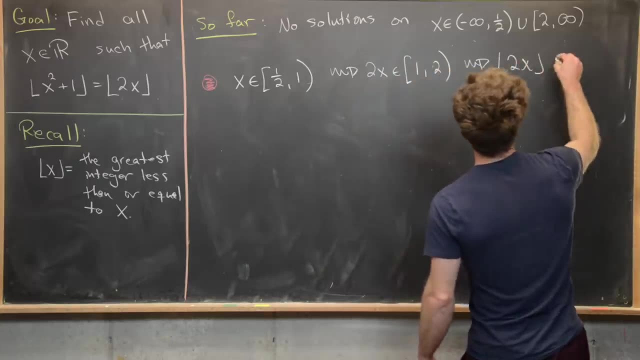 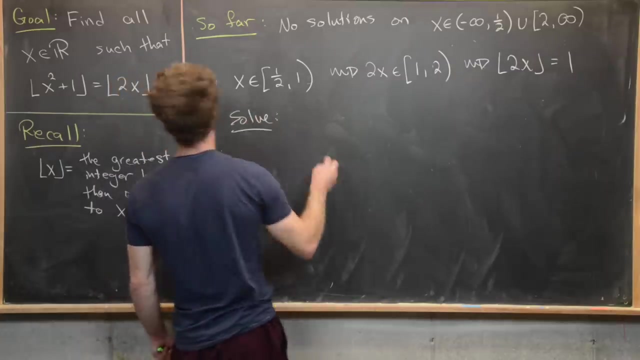 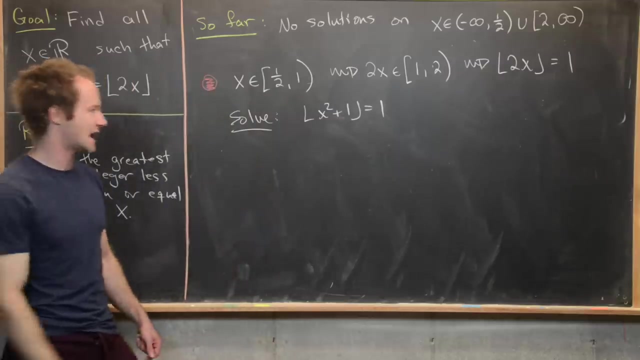 is on the interval one to two, not including two, which tells us that the floor of two x is equal to one, which means what we really need to do is solve for the floor of x squared plus one equal to one. okay, so let's go ahead and do that. notice that the floor of x squared plus one equals. 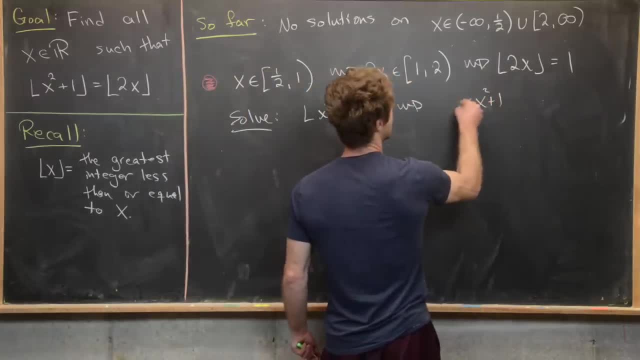 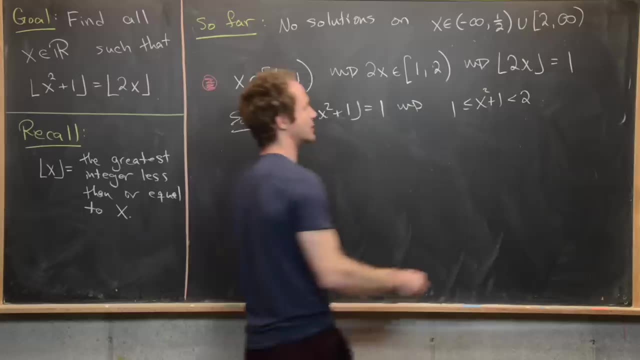 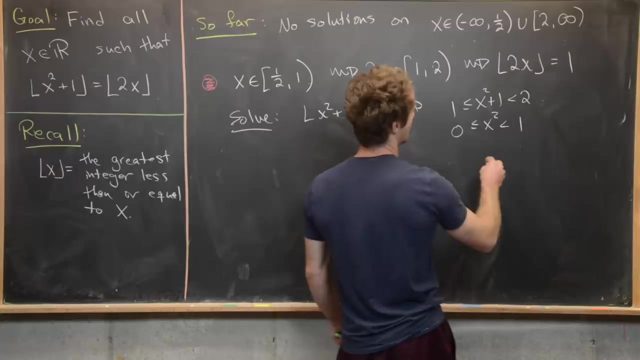 one is the same thing as x squared plus one, being bigger than or equal to one or strictly less than two. but now notice that that means that x squared plus one is equal to one, and x squared plus one is bigger than or equal to zero and strictly less than one, which means that x is between zero and. 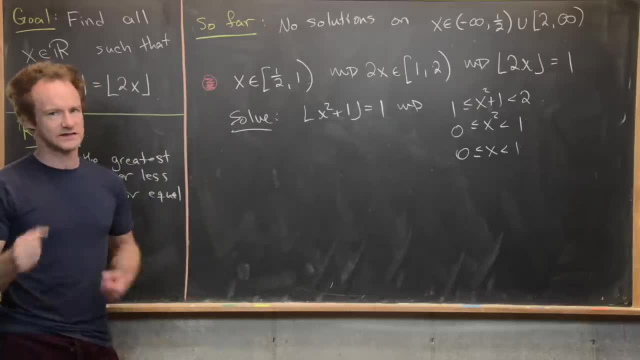 one notice. we don't need to worry about like taking absolute values here or doing a plus or a minus here, because we're already assuming that x is between one half and one. okay, so notice that our original assumption was stricter than what we got in the other case, which means 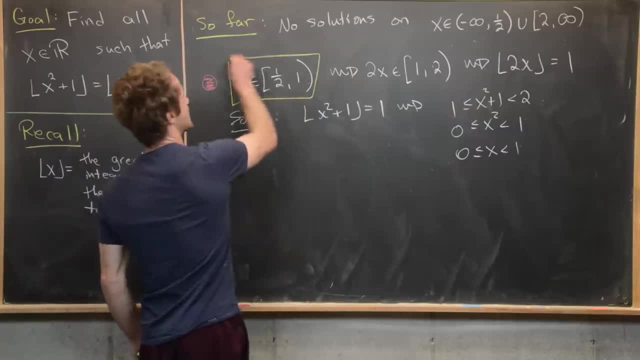 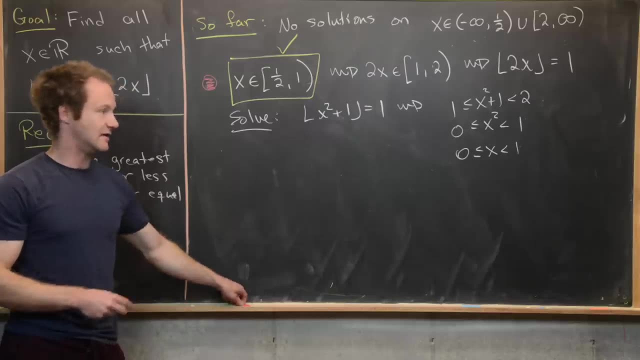 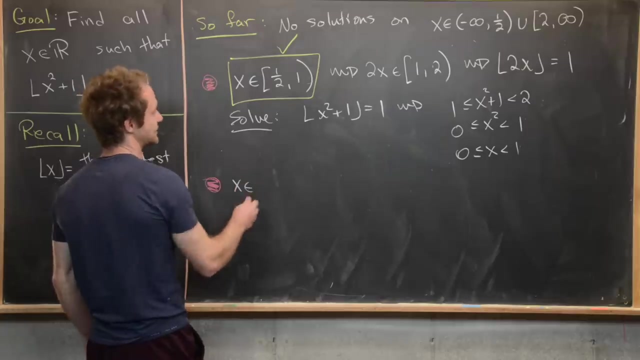 every value of x between here and here is okay. if we had gotten a further restriction down here, then we would have had to intersect, as we'll see in the following cases. all right, let's go ahead and do the next one. so the next one will be: x is in the interval given by one up to three halves. 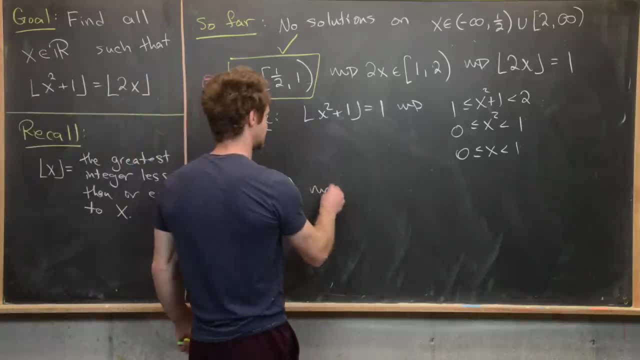 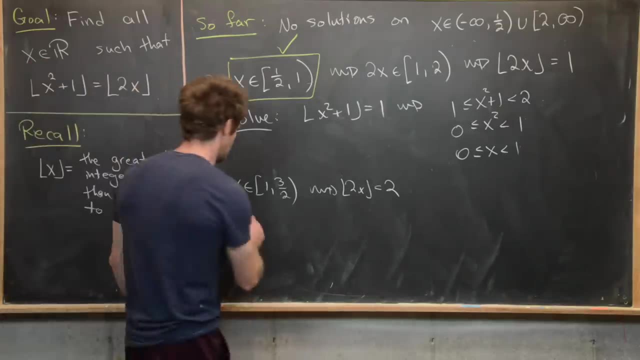 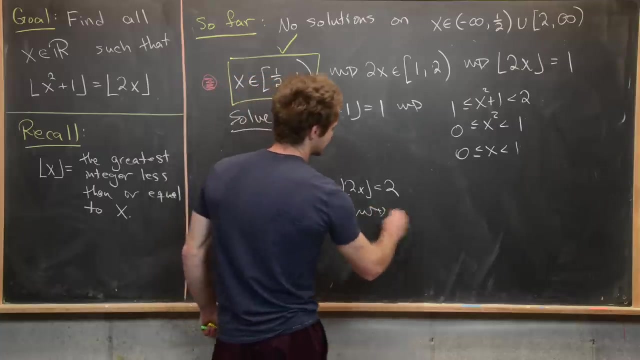 so let's see that means that floor of two x equals two. so i'll skip that step in the middle, which means we need to solve: floor of x squared plus one equals two, which is the same thing as saying that x squared plus one needs to be bigger than or equal to two, but strictly less than three. 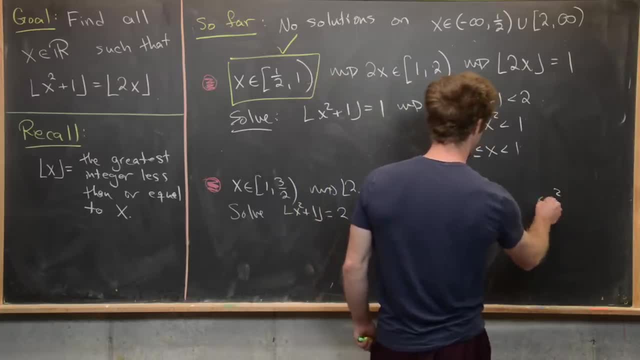 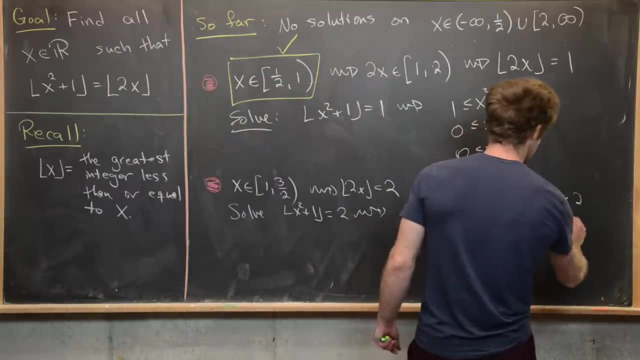 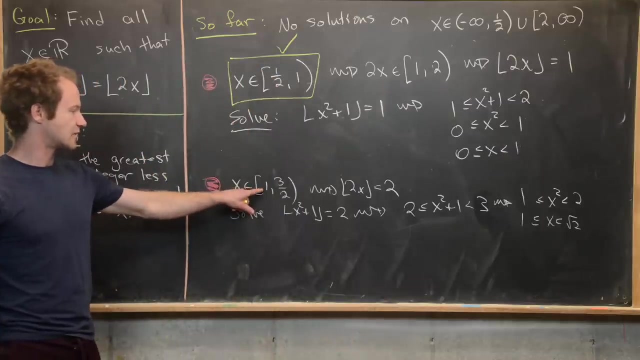 but now notice that that tells us that x squared needs to be bigger than or equal to one, but strictly less than two. but that tells us that x is strictly less than the square root of two, but bigger than or equal to one. Good, So if we're on the interval one to three halves, then we're in fact restricted to this. 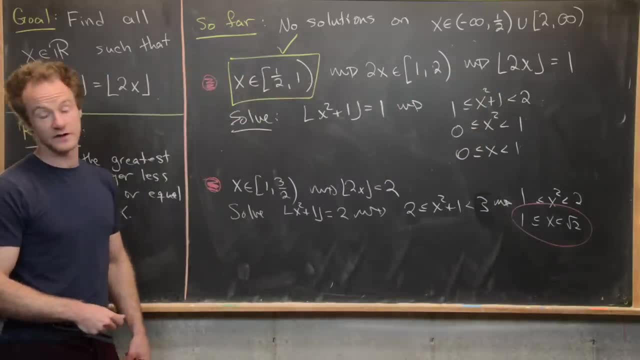 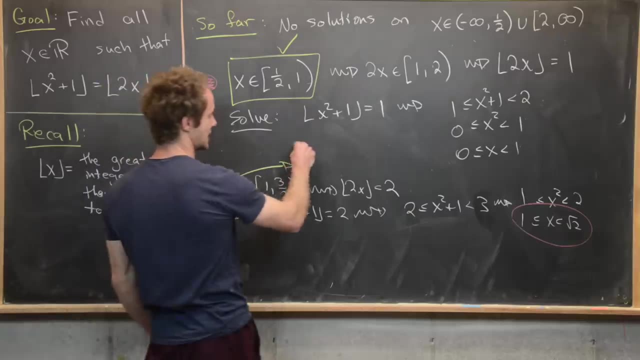 interval one to the square root of three. sorry, the square root of two. So that means that we can reduce this from our starting interval to that interval at the end that we calculated. So one root two. Of course we're using the fact here that root two is smaller than three halves. 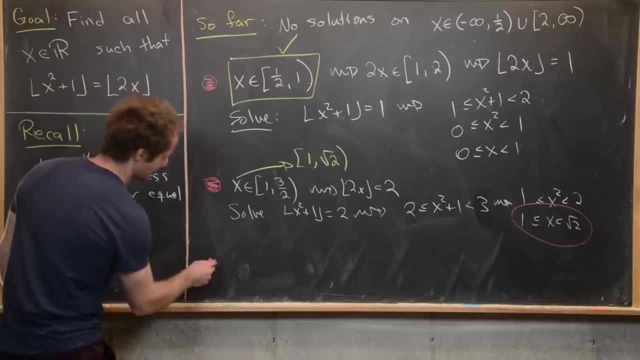 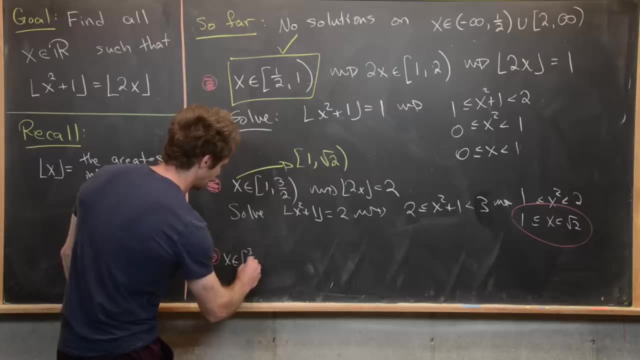 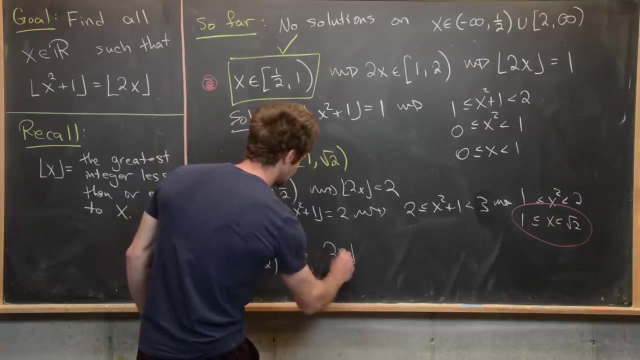 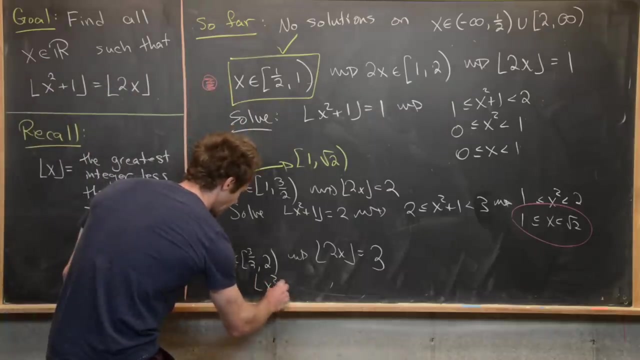 Okay, good, So now the next thing that we want to do is our last case, And that last case will be: x is on the interval. three halves up to two. Good, But in this case we get two. x floor is equal to three, which means we need to solve the floor of x squared plus one equals three. 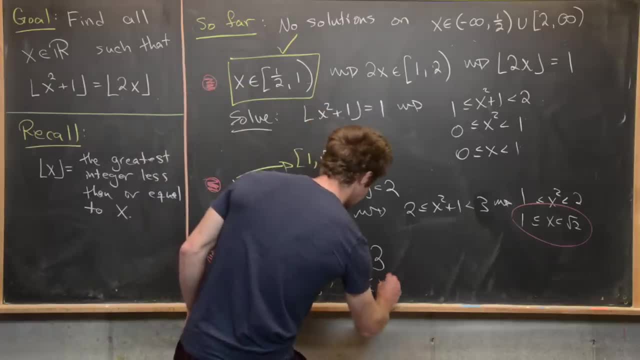 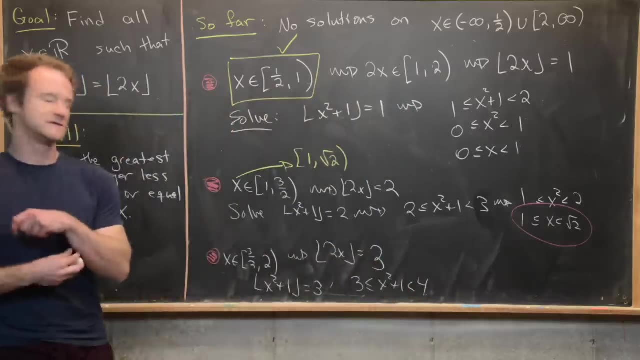 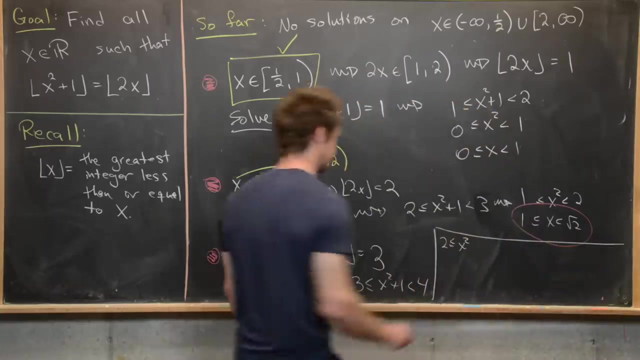 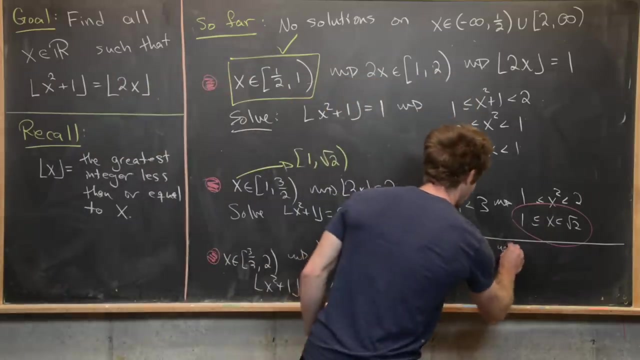 which is equivalent to saying three is less than or equal to x squared plus one, which is strictly less than four. Good, But now notice that that means that x squared is bigger than or equal to two And it is strictly less than three. But now that tells us that x is between the square root of three and the square. 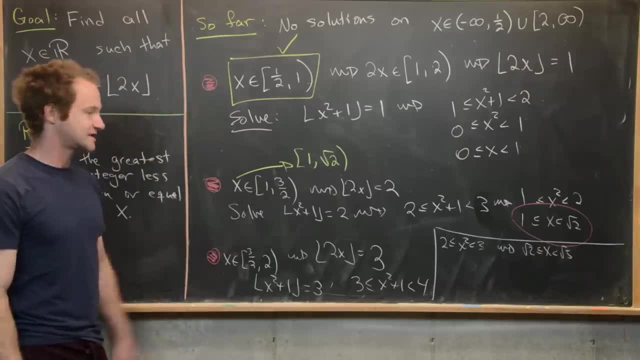 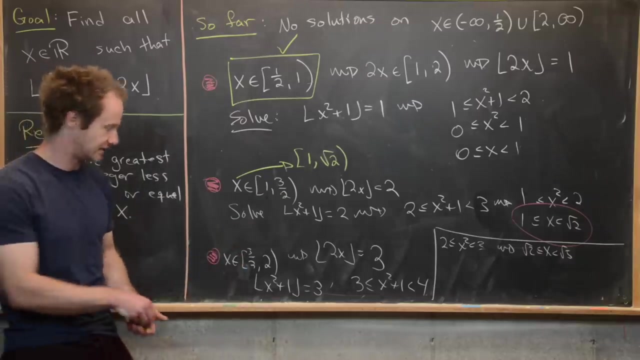 root of two. Great, But now we want to intersect those two conditions, So x being between three halves and two, and x being between root two and root three. Notice that this lower bound is more restrictive and square root of three is an upper bound, is more restrictive. So that means that here we can. 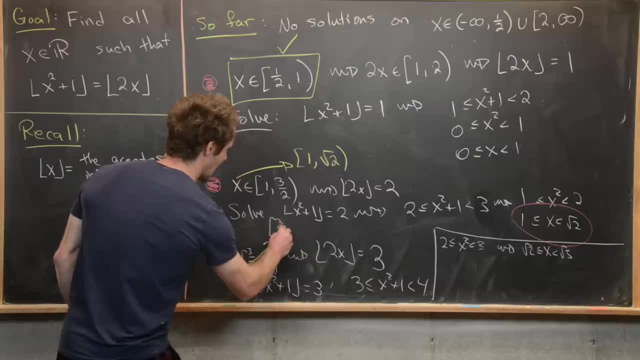 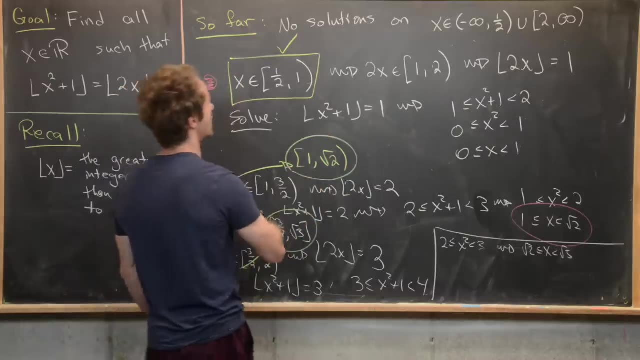 replace this with three halves up to the square root of three. So now we found our three intervals- this one, this one and three, And now we want to intersect those two conditions. So x being between three halves and two is going to be x squared plus three. So we're going to have to do this.